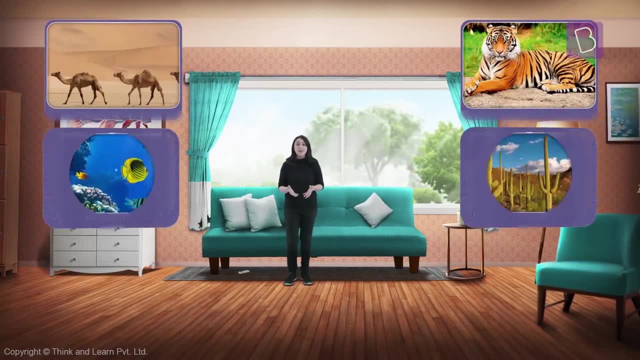 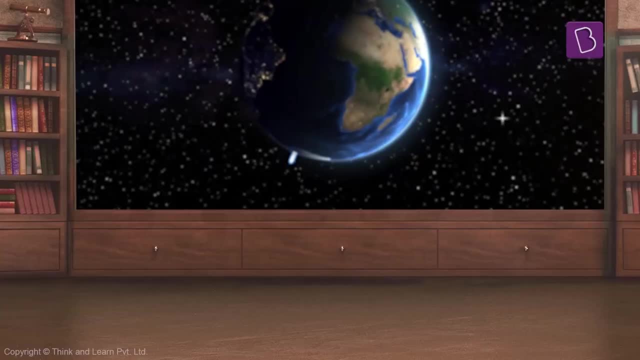 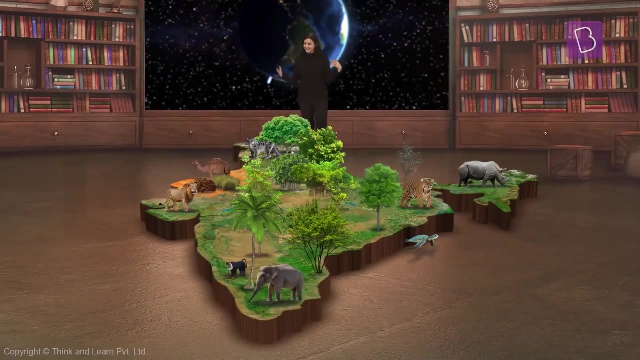 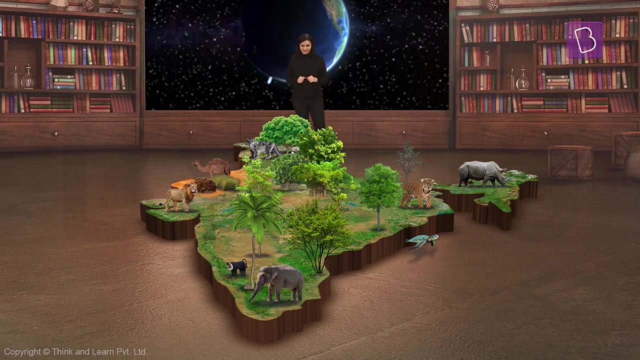 Like the elephants, each animal and plant in the country can exist only in the kinds of places that they do exist, And this is India. Now, these are the kinds of plants and animals that you find all over the country. Nice, Okay, let's take a look at the Himalayas. 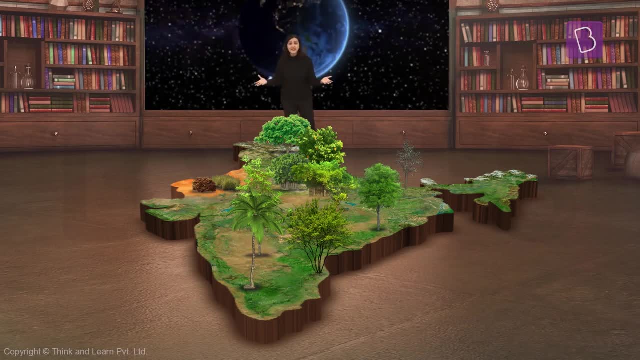 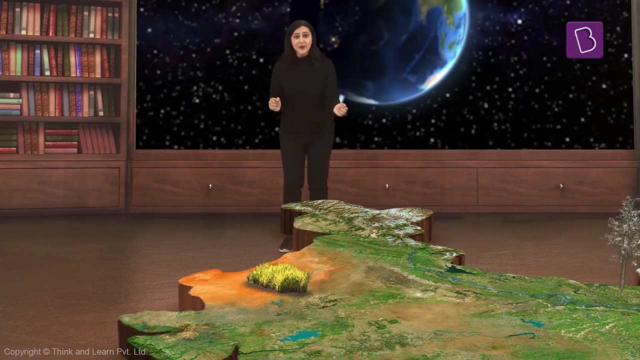 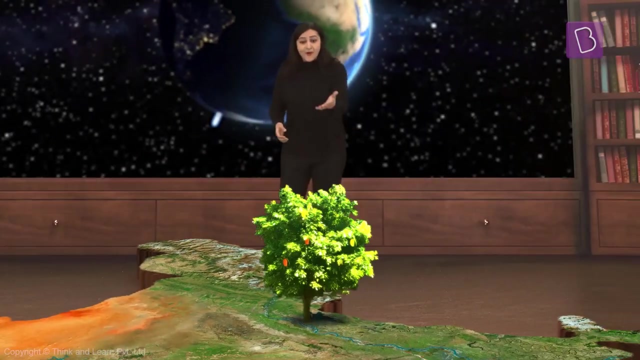 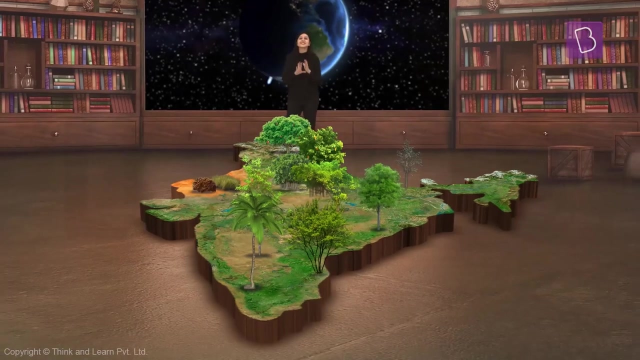 All the plants in the country, So many different kinds. We've got large grasslands, We've got bushes, We've got shrubs, We've got trees, So many trees. We've got neem, apple, mango, coconut- Oh, I love coconut, People banyan- The list is just endless. And all these trees. 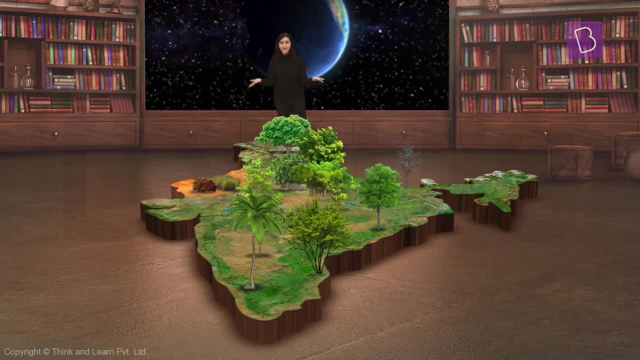 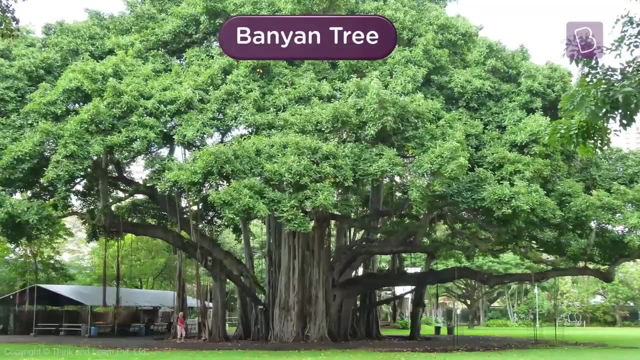 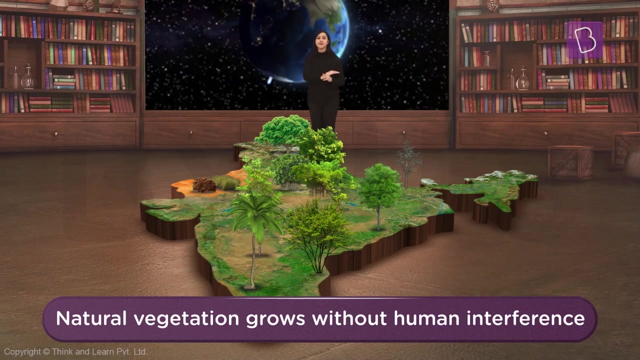 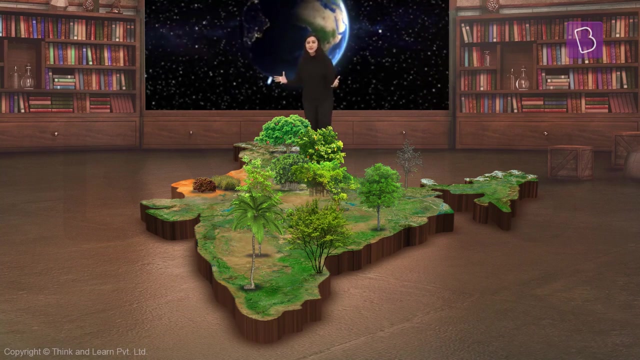 are different from each other, See, some of them have less leaves, Some of them are taller, Some of them are wider, But they are all natural, though They all came up without any human interference. This is the natural vegetation of India, And we have all this variety in our natural vegetation because of our brilliant climate. 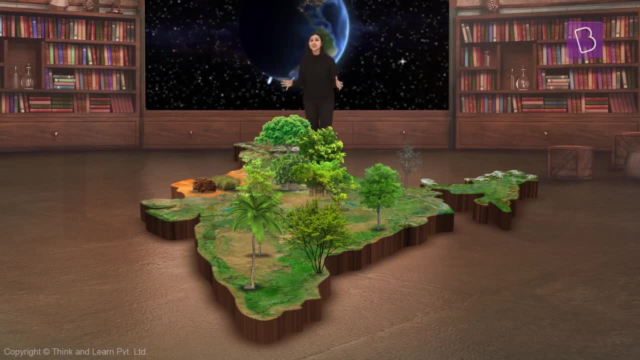 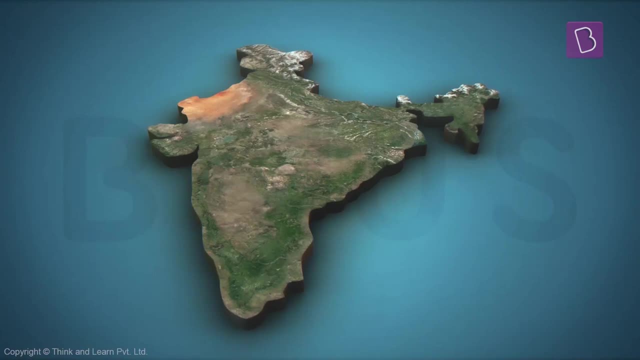 So let me take you through the different types of plants and animals that we find in the Himalayas, Different types of natural vegetation in the country, and show you. Look at the physical map of India, So let's look at all the different kinds of landscapes that we've got. 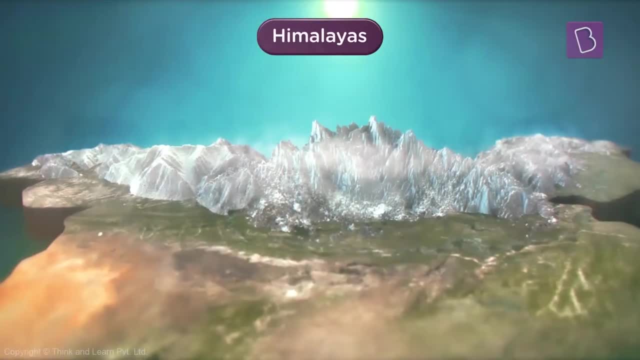 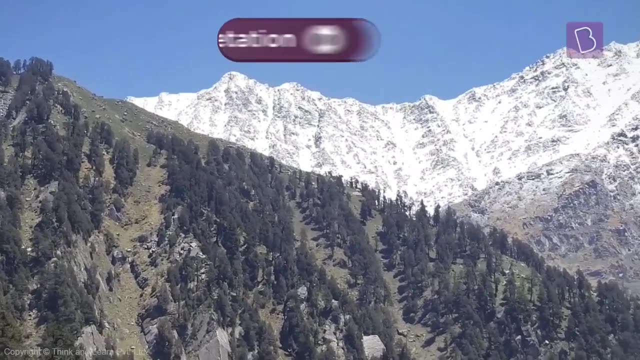 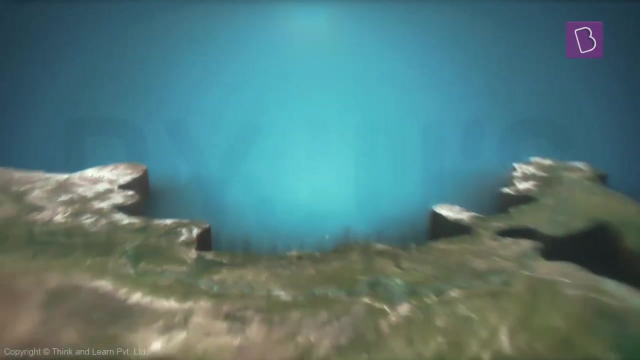 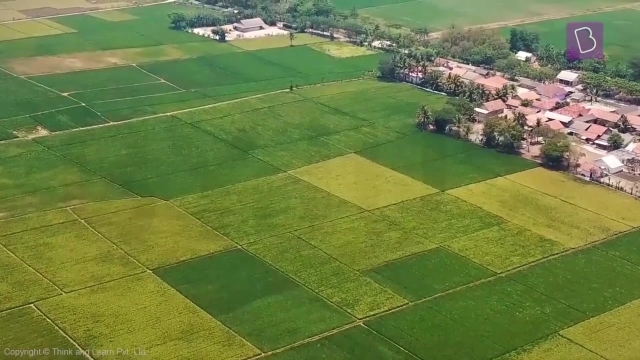 So up here we've got the Himalayas, Huge mountains capped with ice, where the climate is extreme and brutal. Now the vegetation here is thin and distributed. It's mostly ice throughout. Then we have the Gangetic Plains right below the Himalayas, filled with farmlands and crops. 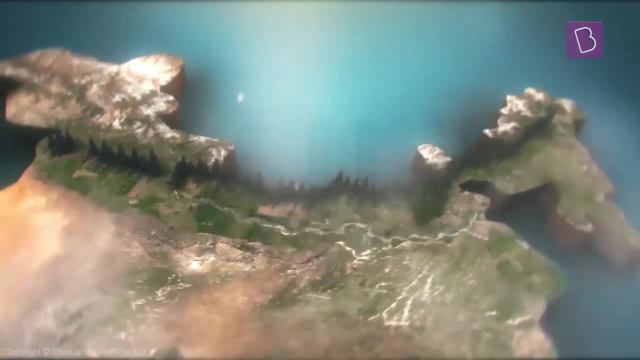 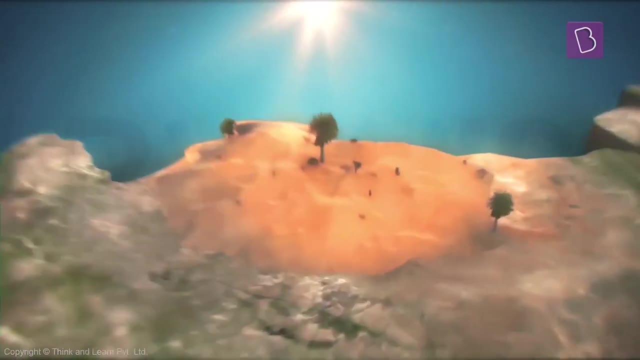 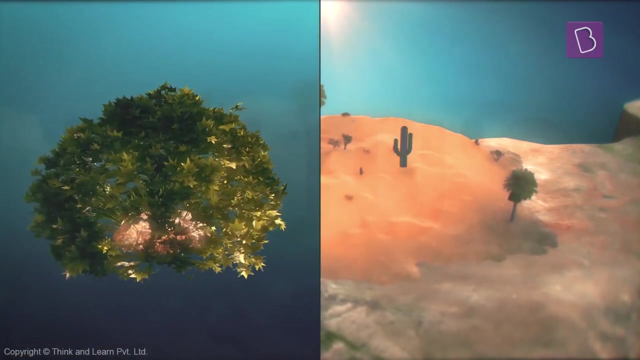 Now these are the Northern Plains, formed by the deposit from the Ganga and the Brahmaputra, In complete contrast. over here in Rajasthan, where we have the Thar Desert, you will find only thorny bushes and cactus. You can see everything from Jiangsu territory to the South бог, to the north vorوب, to the east border. You will never experience a two- phenyl lead vegetation at all. You can see what beautiful it will be. People should be made present at times.